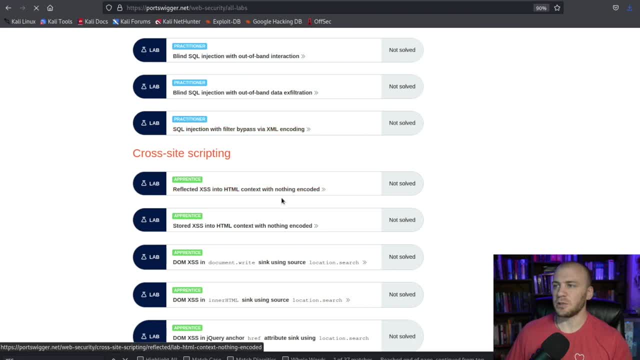 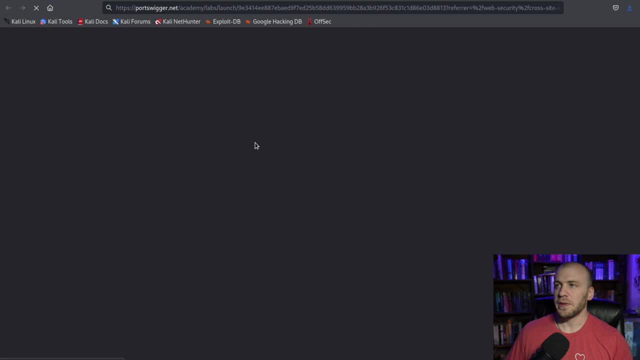 more difficult, but still, nonetheless, it's still pretty easy. So we'll go ahead and open up that lab. We'll access the lab right here and this is going to go ahead and load, And it has loaded finally, So you'll have this search bar right here. I like to open up Burp and go ahead. 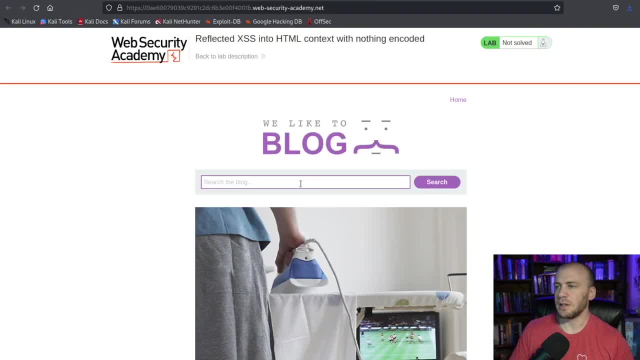 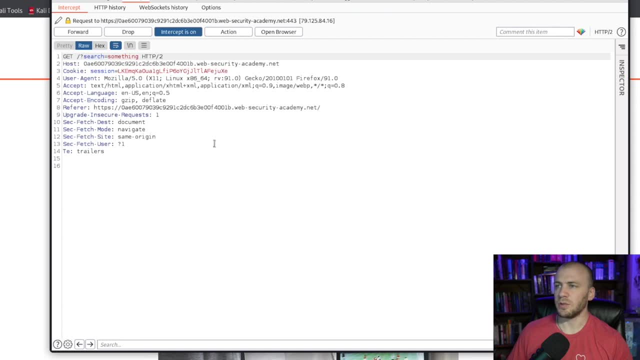 and turn the proxy on and just type in something just like this and hit search, And so we have our search right here. I think it's a control R, since it's to repeater, and we can shut that off, And now we can go ahead and open up the lab, And so we have our search right here, And so we have our. 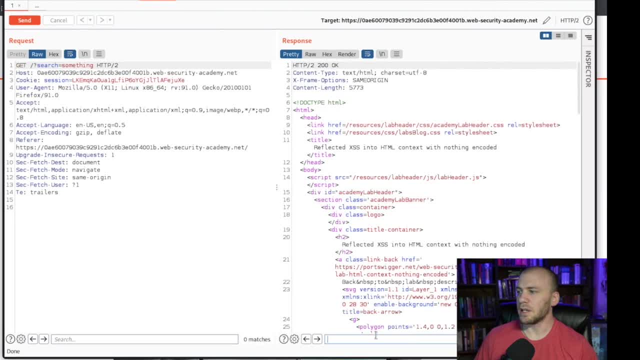 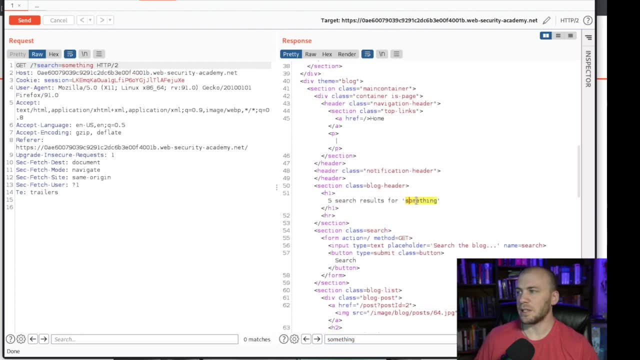 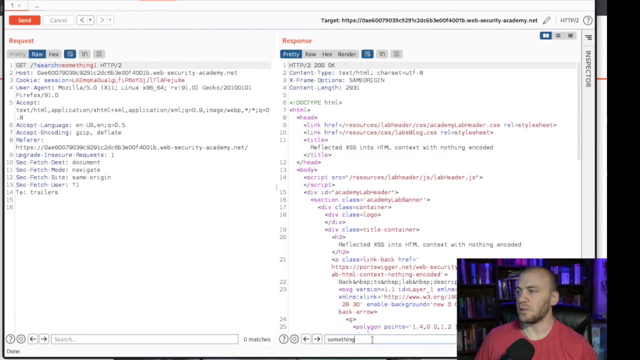 request. I come to this little search bar down here and I type in something and it's going to tell you, inside of this H1 tag, what we type in right here is going to show up. So we can type in, like something one and send this And you're going to be able to see that something one pops in, right. 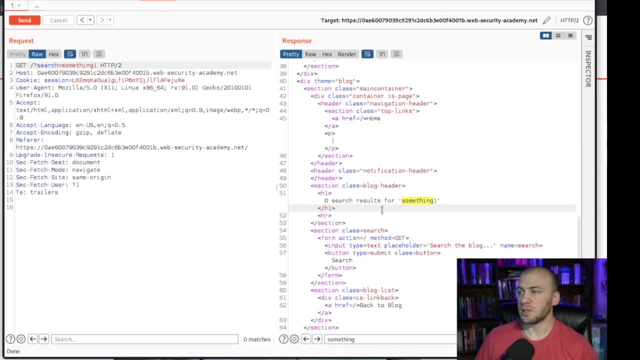 here, inside this HTML, which this is going to be super simple to inject into, because you're just inside this H1 tag right here. You don't even have to break out of anything. So we can go ahead and do this from here. You can type out just a normal script tag with the alert one, and then we 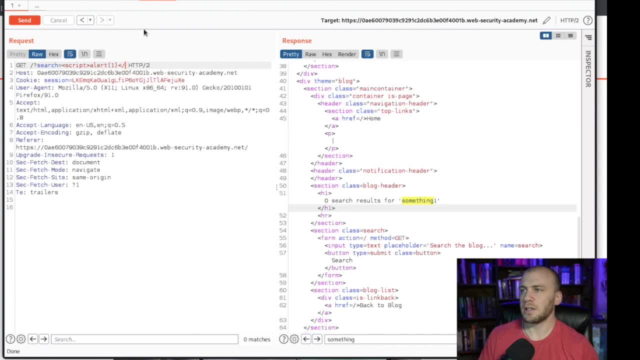 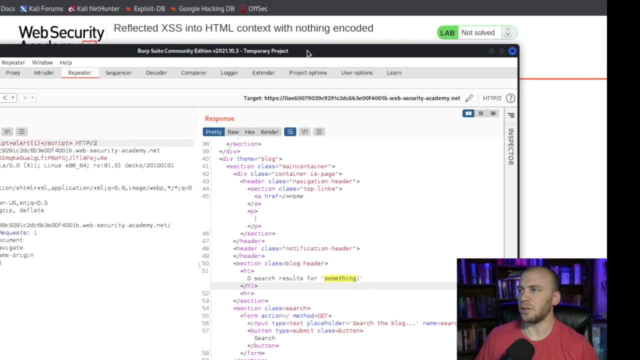 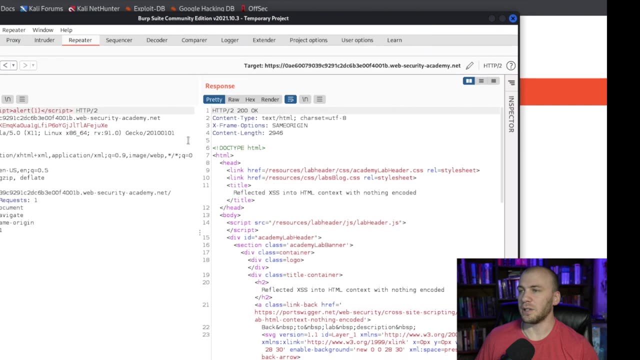 can close this off, move my mouse just like this, And now if we send this, this should send to the back end and just say: should pop up with our solved lab right here. So we can send this and it changes to a solve. but that doesn't really help us. So if I do something like this, 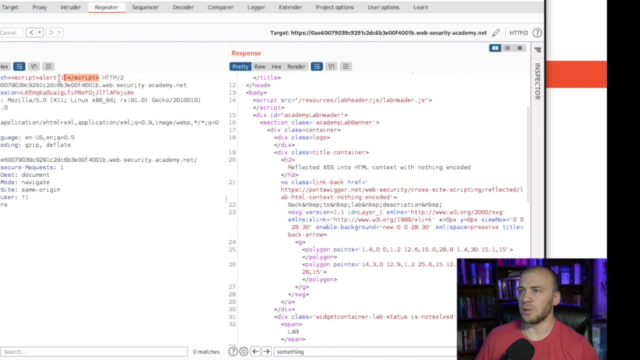 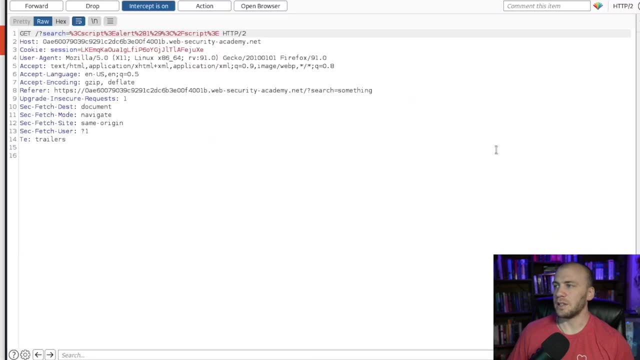 I like to see it over here, but what I usually would do is I would take this right here and I'd come back to my proxy, I would turn the interceptor on and I would send something like this over here, So the way I can see exactly what is happening, let's send this to repeater and turn that off. 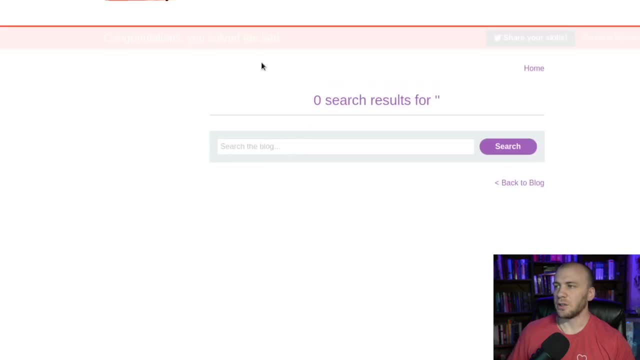 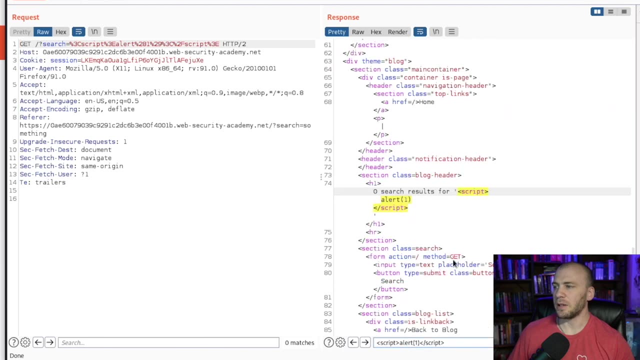 But then also you're gonna be able to see this pop over here. So there is another way to look at this, but I think burp is probably the easiest way to see this. So if we send this and then we type our payload in right here, 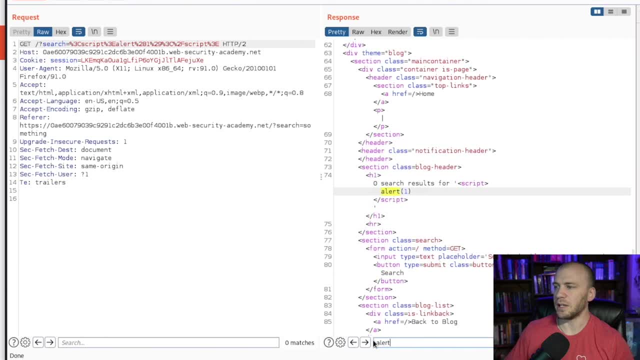 you're gonna be able to see right here, So we could just type in alert down at the bottom and you can see your script tags. Now this is gonna be really important in the next one, And I'm gonna show you why it matters that we can find it inside of the HTML. 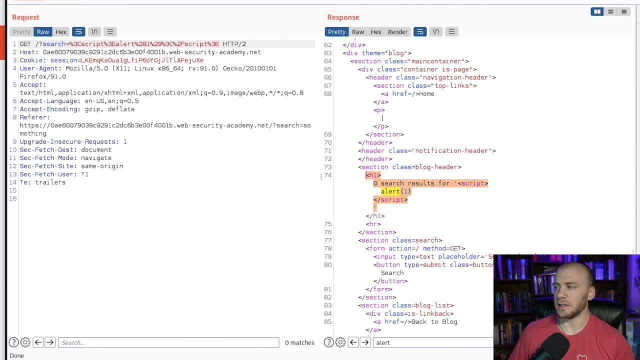 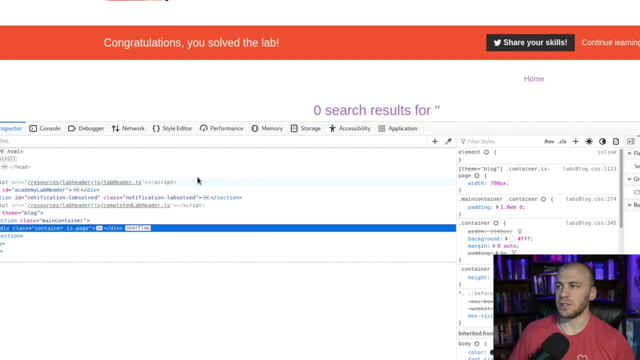 because sometimes we're gonna need to break this and it's gonna take some debugging. Some people I know like to do this with the inspect tools over here, So you'd open this up and find where you're searching for over here, but I find it easier to look inside of burp, So let's go ahead. 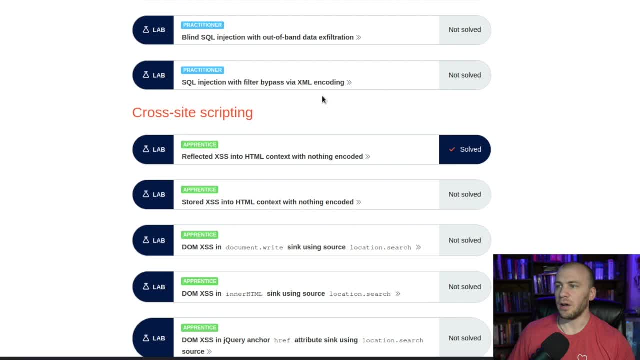 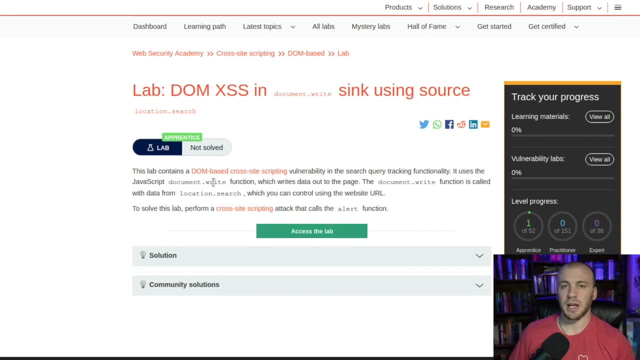 and come back over here to our options, and we'll go to this one right here, And I think this one's going to be a little easier to understand why I look in burp, specifically because we're gonna have to break the HTML in order to get this to inject for us. Okay, so we're brought back to 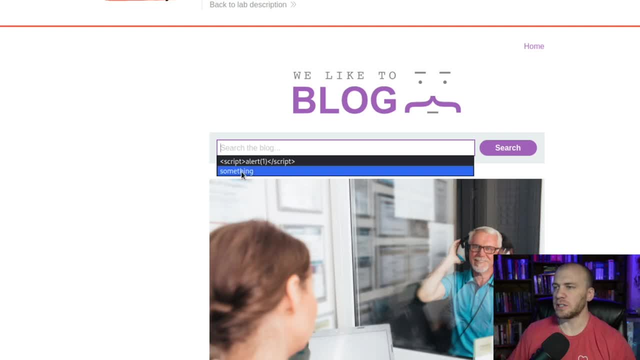 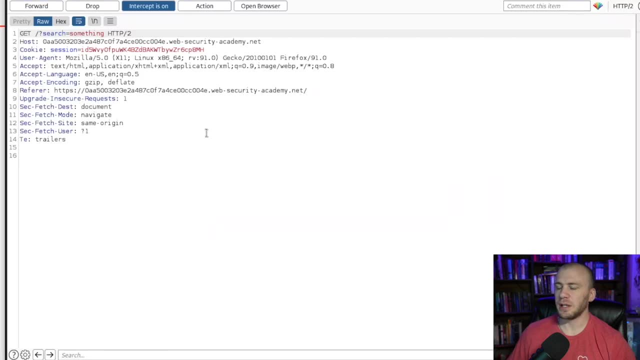 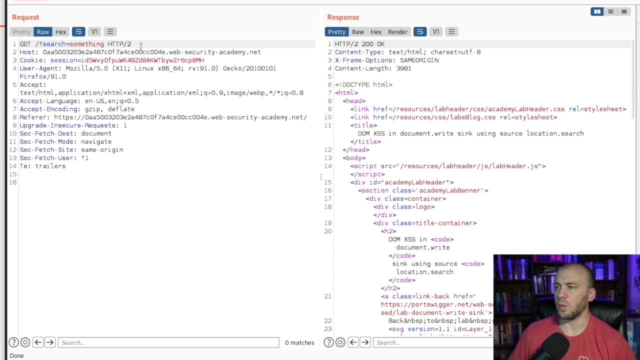 the same search bar and what we can do is just like we did before. we can just say something: Come back to our proxy, turn it on, search it, and we can send this to repeater. turn the interceptor off. and we're going to want to look at this request. we want to know where our word search. 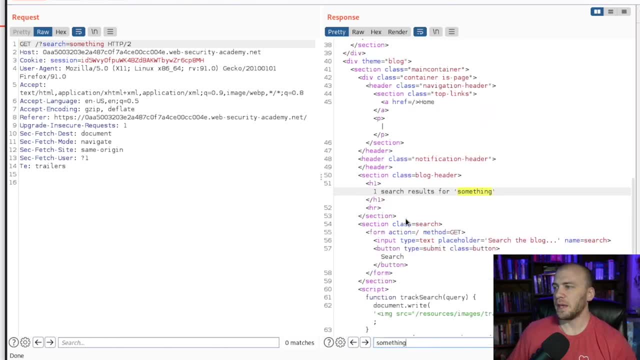 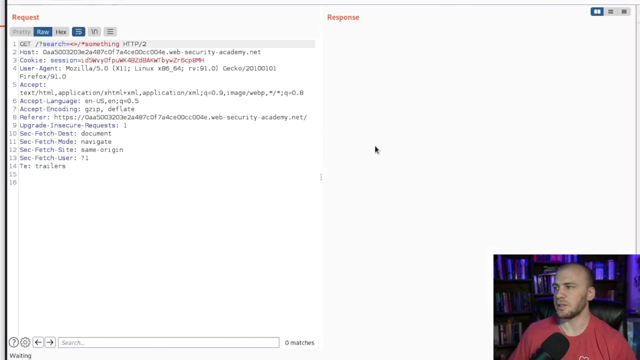 that we inserted is at, so we can type in something and we can see that it is right. here it's still inside the h1 and let's see what happens if we add in some special characters like this: just throw some special characters in there and see. if it it does, it changes those for us. so we're not 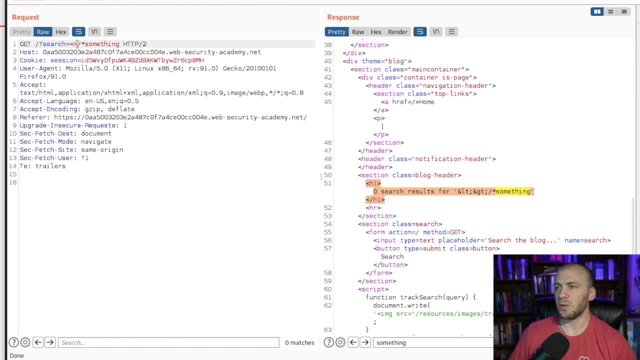 able to break the html right here. so this is something that you're going to want to do when you're looking for cross-site scripting is put in some special characters, so you know what you can use and what you can't, and i'm sure you can go out to github and pull open a github page. it's. 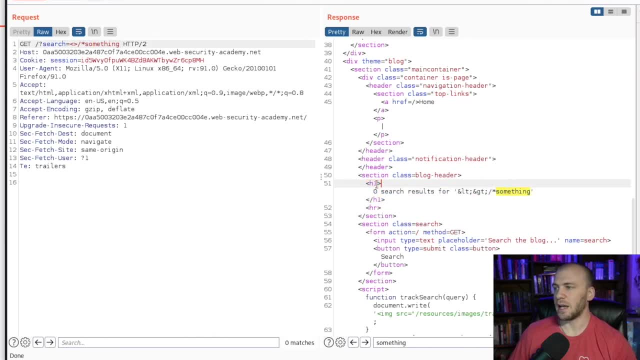 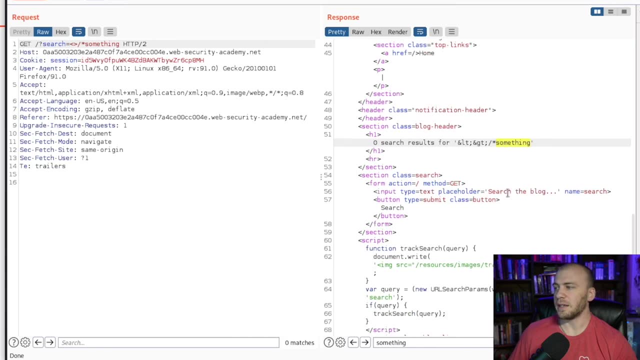 just going to have the special characters in here. so what is happening is we're able to put this in here. it is going to change our special characters so that we can't break like we were right here and then down here it looks like our query is being changed into a function, so this is going. 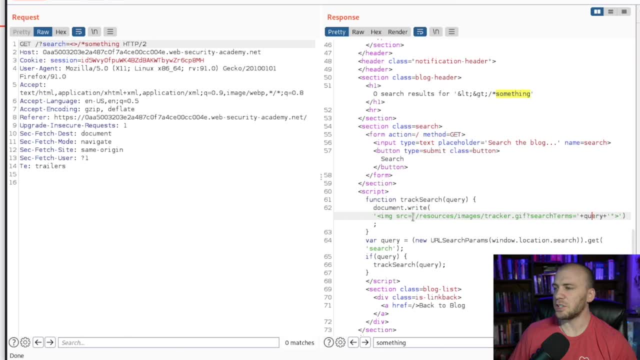 to be our a query and we're going to see if we can inject right here. so we have this javascript, so we got this document dot right and it's going to go to this image source. we are going to be breaking this query right here so you can see we're inside of an image tag and our query is right here. we. 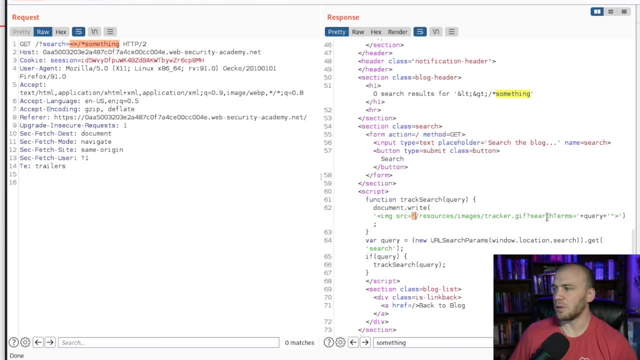 have a source and we have a double quote, a single quote and then there's another double quote over here. so if our query comes in right here, we can break this with a double quote. so let's see what happens if we just go and type in a double quote and we'll just send this and then go. 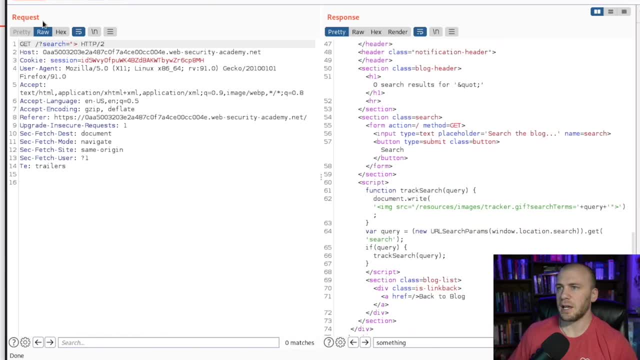 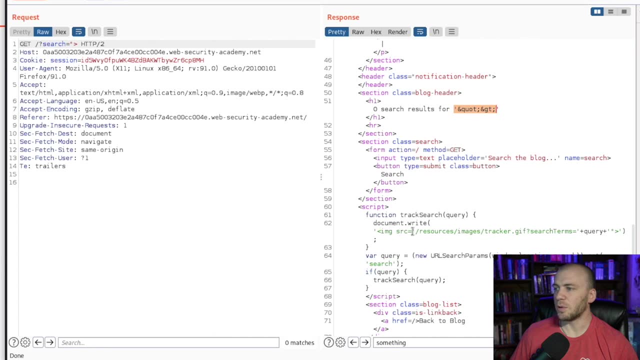 back and look and see what happens. let's try and close off that image tag, because that doesn't look any different. we have our quotes right here, so we should be able to do a double quote and then a single and then close off this image tag inside this query right here, and then we should be able. 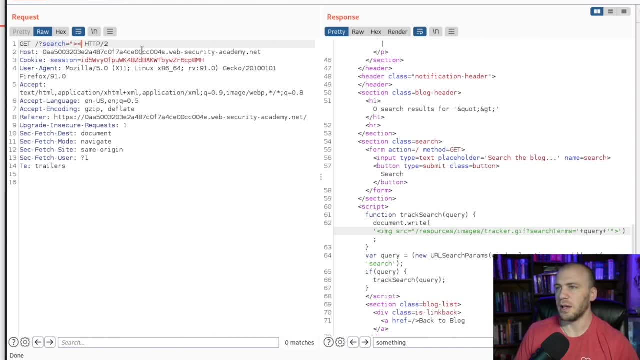 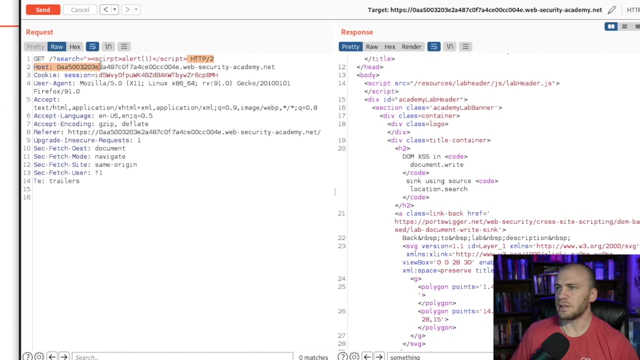 to put in a payload, so we should be able to use the same payload that we did before. so script alert one and then we can close this off like this and send it see what happens. it says: not solved over there. let's copy this and see what happens if we take this over here and we hit search. 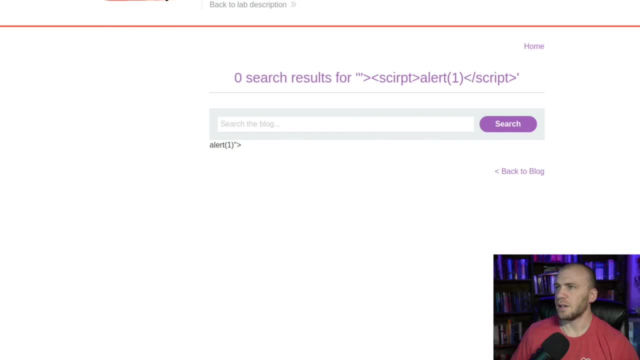 it tells us that it does not solve and after looking at this i can see we have a typo. so let's come back over here, let's actually copy this and paste it back in here, because we see something popping up down here, so we know that our tags have a change and i'll show you what i mean. so if we 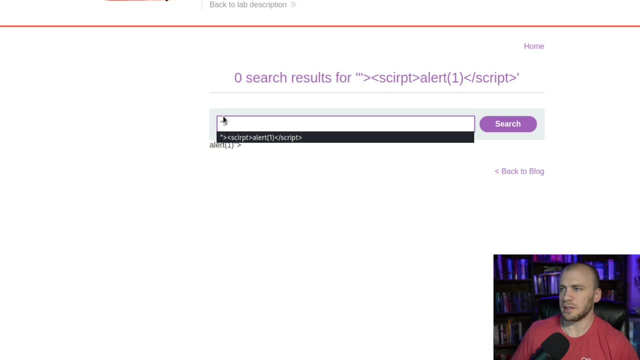 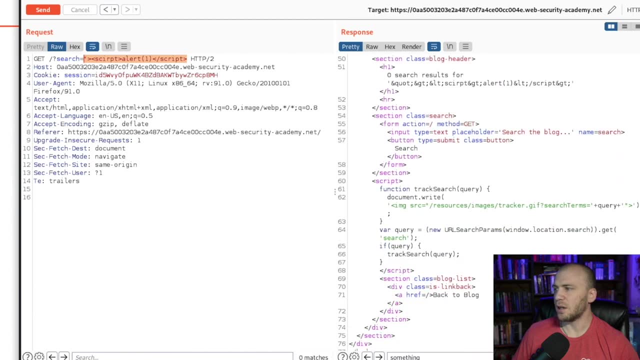 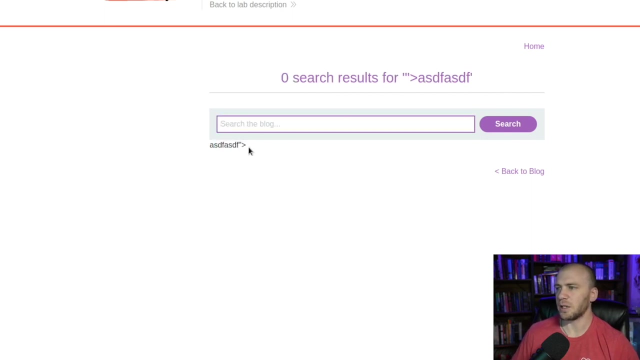 come in here and we close off what we saw previously with this image tag. right here we close this image tag off and then we can put something in here and it is showing up down here. so we know that we're able to break out of that image tag because the html shows up. so now we can close, break out of the image tag. 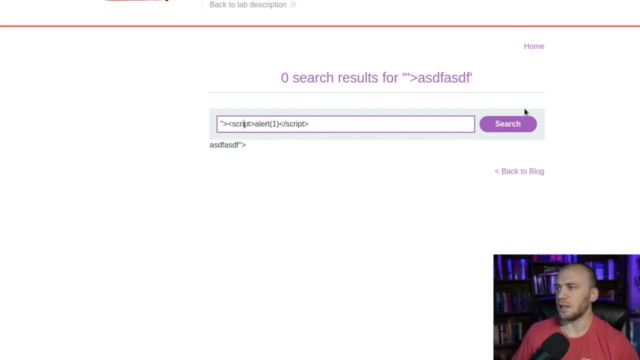 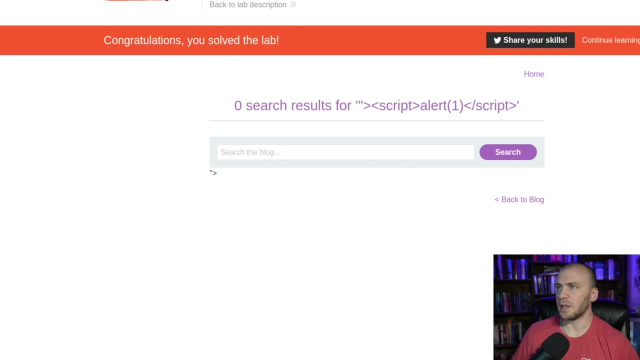 we'll just use this and we'll come over here and spell this right and hit search and it should work for us and it does. so. this is how you would solve something where you're able to look at this right here and see we have a double quote right here and we're able to use our query and break out.